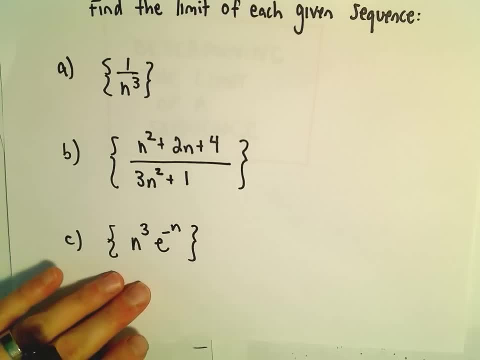 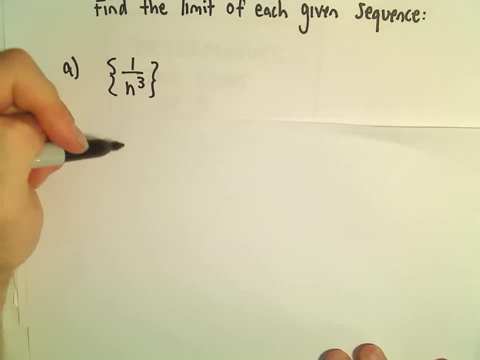 Alright, in this video we're going to look at determining the limit of a few different sequences. So in part A we have the sequence associated with 1 over n cubed. So what we'll do is, again, we just take the limit, as n goes to infinity, of 1 over n cubed. 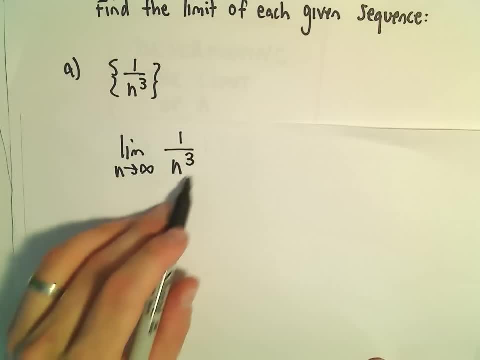 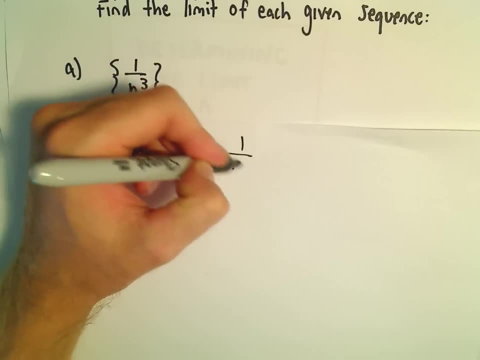 Well, as n gets really really really big, the denominator is going to get really really really big. We're going to have 1 over a very, very big number. So 1 over a large number gets arbitrarily close to 0.. 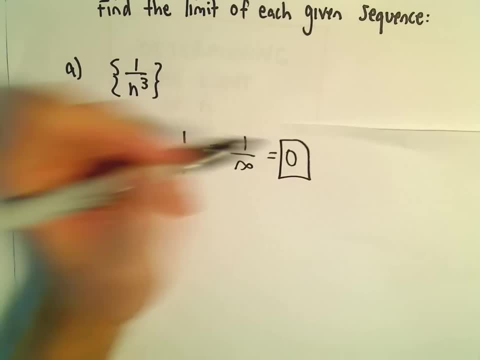 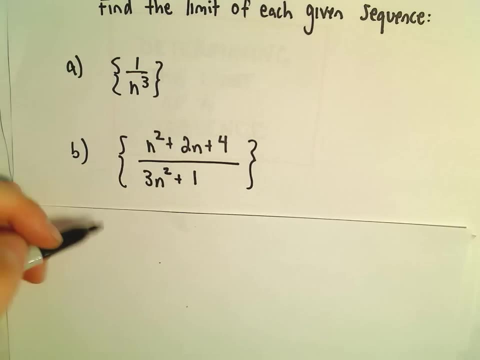 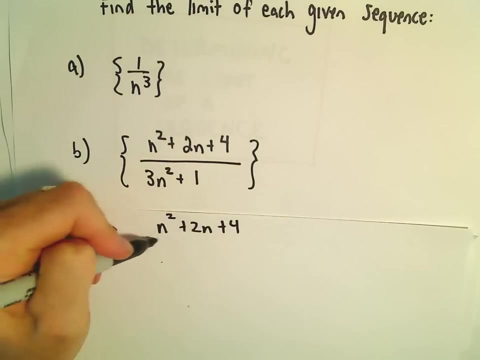 So the limit of the following would just simply equal 0.. Part B: same thing. we'll just take the limit as n goes to infinity. So recall the shortcut. if the degree of the numerator is equal to the degree of the denominator, 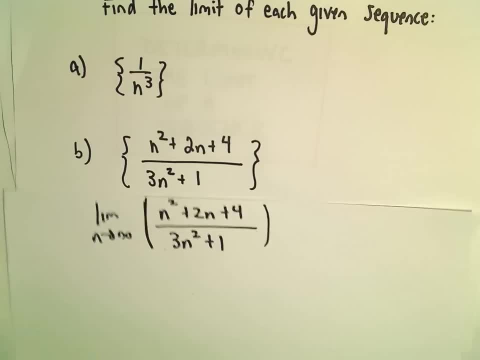 we just do the ratio of the coefficients, So I can just simply look at this and say: well, this is a denominator. This is 1n squared and 3n squared. The degree of the top equals the degree of the bottom. 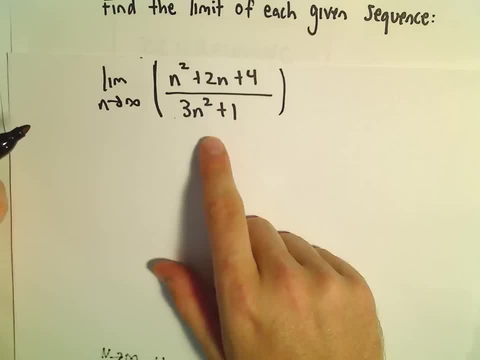 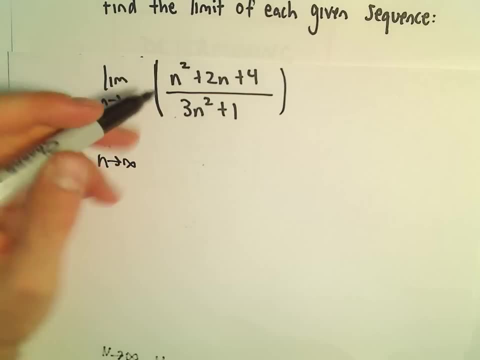 We'll get 1 third. It's a very useful little shortcut to remember when you do sequences in series. But again, kind of to show it with a little bit more work, we can divide everything by n? squared. So n squared over n squared is 1.. 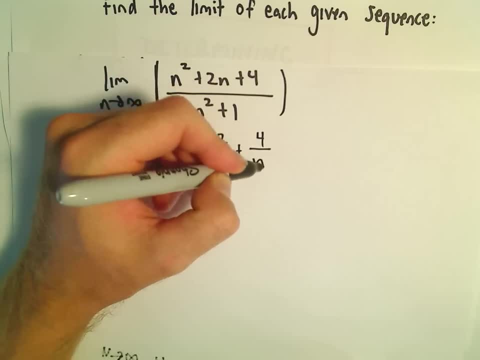 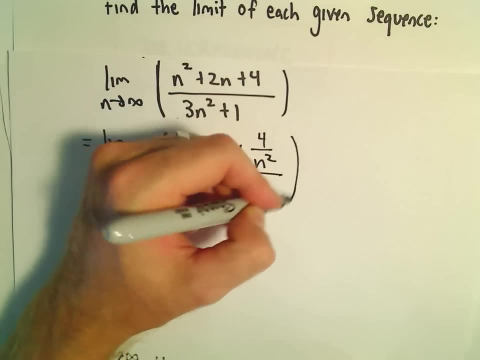 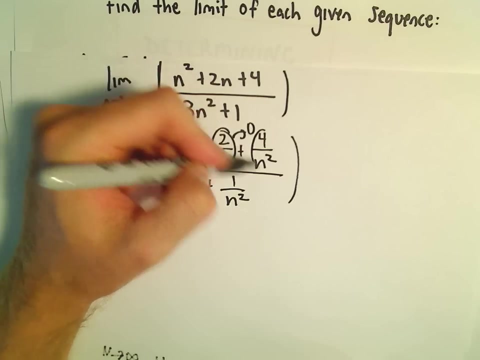 2n over n squared will be 2 over n. Then we'll have 4 over n squared, 3n squared over n squared is 3.. And then 1 over n squared, And again the idea is: now it's more clear, because as n goes to infinity, this term will go to 0.. 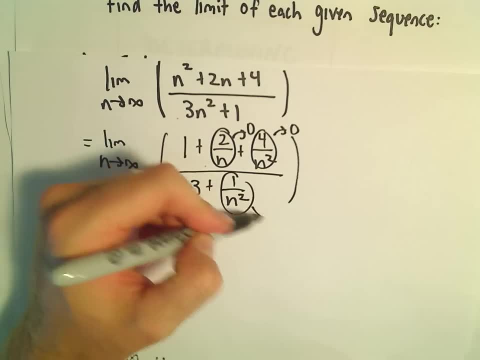 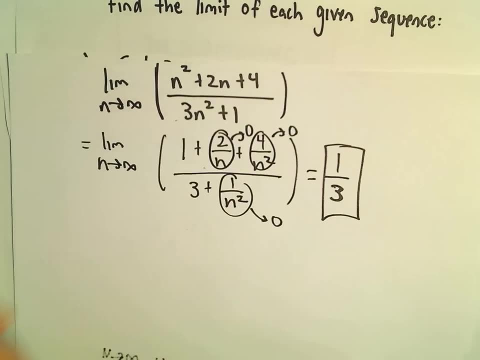 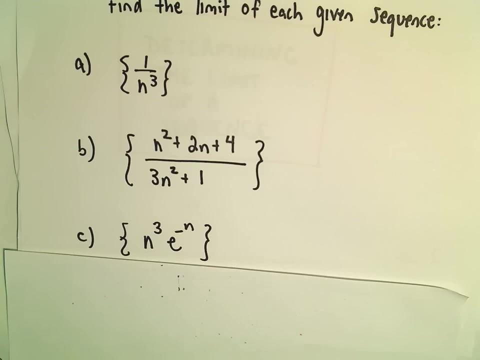 The 4 over n squared will go to 0.. The 1 over n squared will get arbitrarily close to 0.. So again, we're just left with 1 third as the limit for the second sequence. Last but not least, here we have n to the third times, e to the negative n. 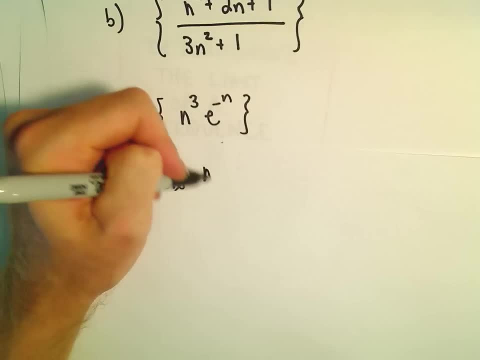 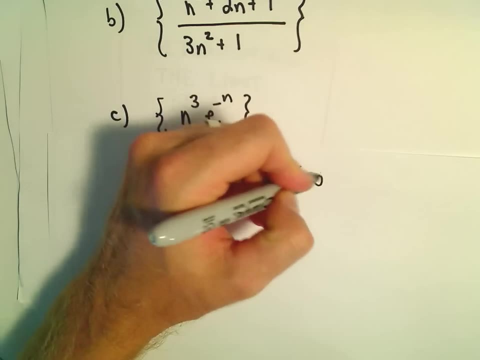 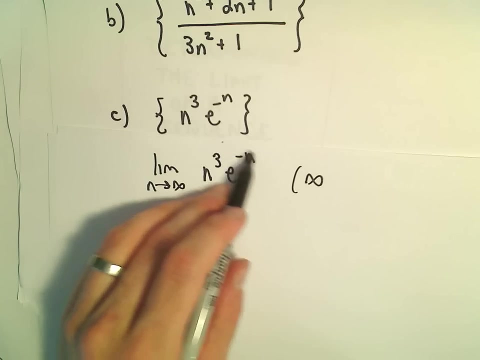 If we do a limit as n goes to infinity, notice we'll get you know, as n goes to infinity, n to the third will go to infinity, But we'll get e to the negative infinity. And if you take e and raise it to a quote, unquote big negative number that gets close to 0..